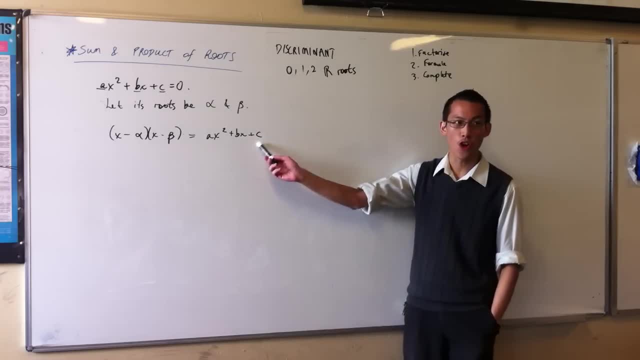 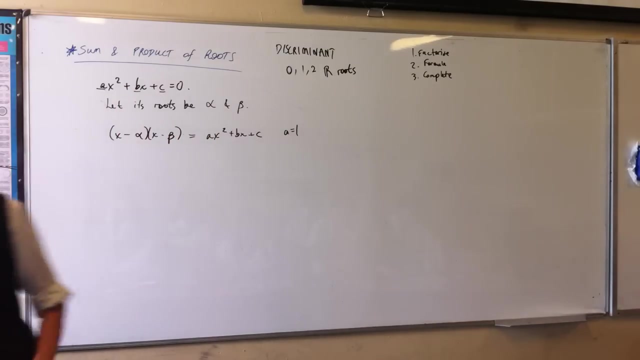 Almost. This equation can only be true when a is equal to 1.. Why? Because if you have 1 coefficient of x, if you open up the brackets, it's going to be x squared. Good, good, good. So in case you didn't catch that right, 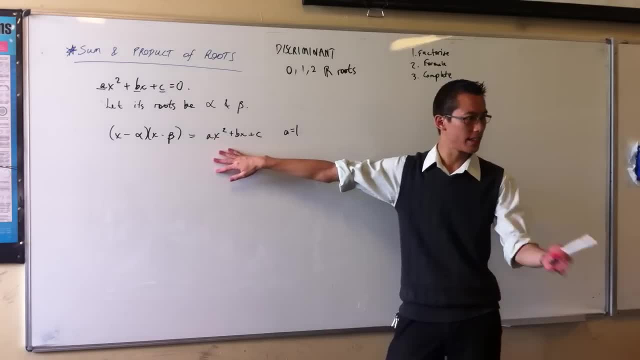 if you have a look on the right-hand side here, right, it's like you've collected like terms and it's finished. All the like terms are gathered together. All of the x squareds are here, all of the x's are here and all the constants are here. 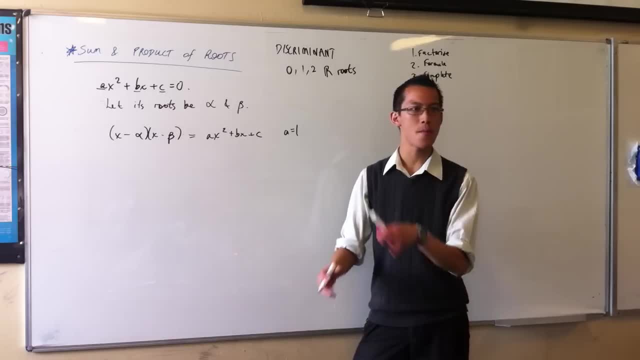 Okay, Now, when you look at this, no matter how you expand it, no matter how you rearrange and do all kinds of weird stuff right, you're never going to get an a out in front of your x squared Right. 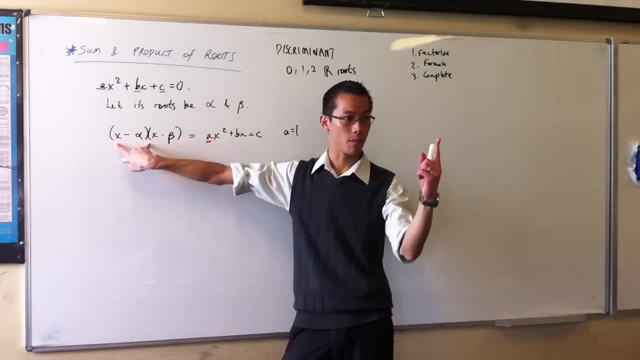 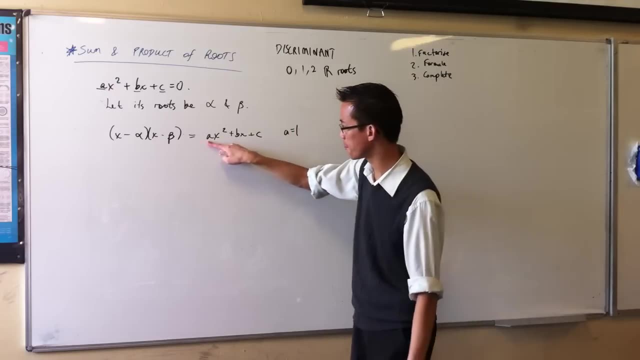 Because all of the x squareds- well, there's only going to be one of them, right, because they come from these two terms. Okay, So this line only works in this case, So I want to fix that right. 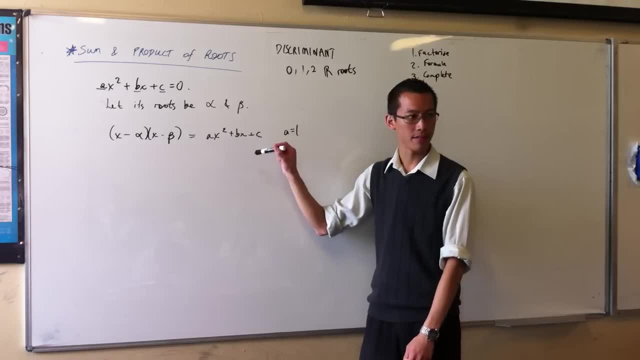 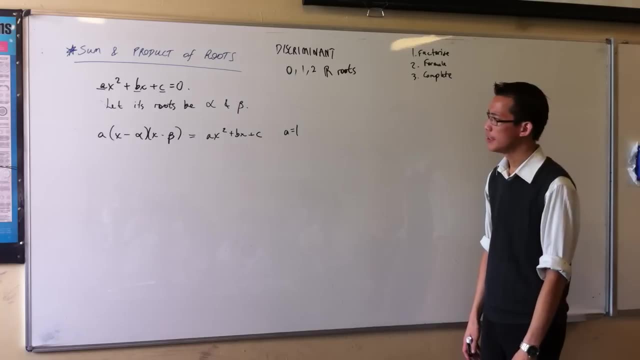 So what I'm going to do is, if I want a lots of x squared on both sides, I'm going to slap an a on the front. Okay, Are you content with that? Okay, now this is actually going to work. 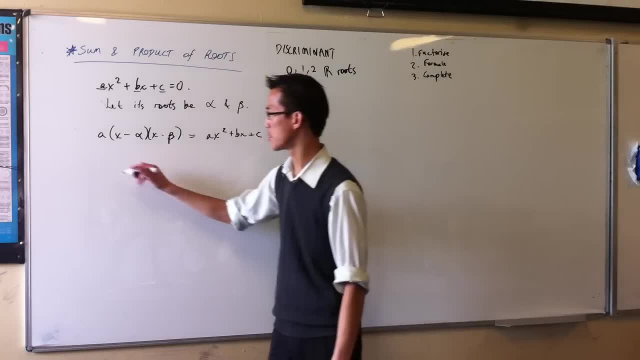 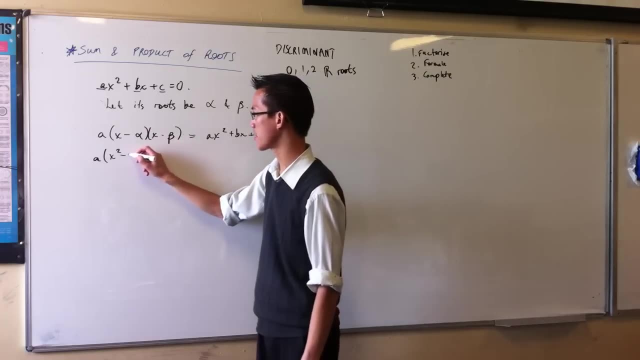 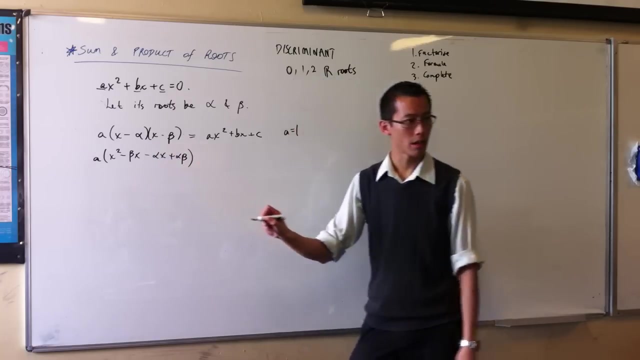 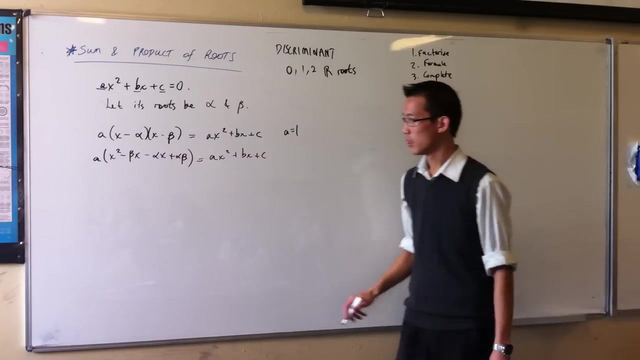 So let's expand this out and see what happens. What happens when you expand this? I'm going to have x squared a squared minus beta, x minus alpha, x plus alpha beta, Is that okay? You see that That's ax squared plus bx plus c. 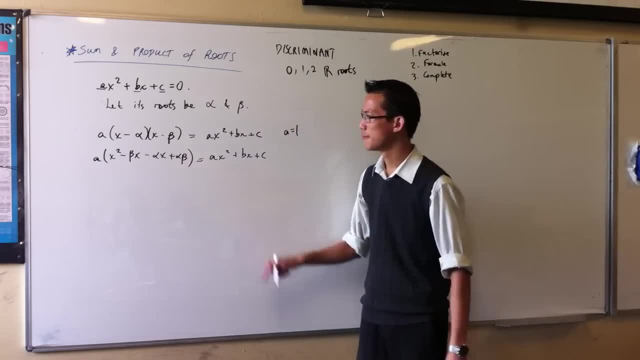 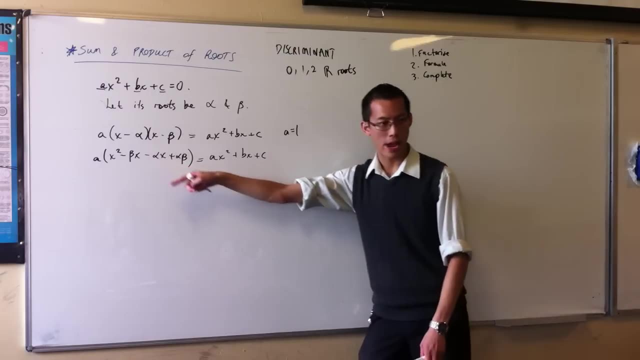 So let's see what I got here. This is a bit of a mess, So is this? What could I do here? Now you've got two options. I think You can expand that out with the a right, or you could take the a over the other side. 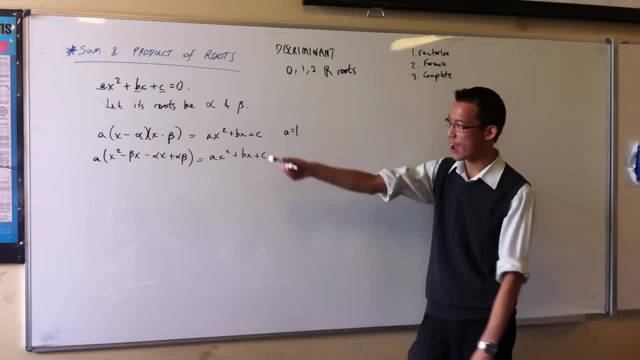 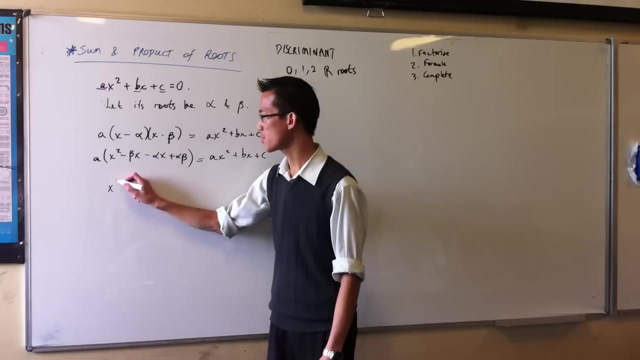 Okay Now, I think either way would work, but I think if I take the a over this other side, the results we're after will be a little more obvious. Okay, So I'm going to divide everything by a. Is that all right? 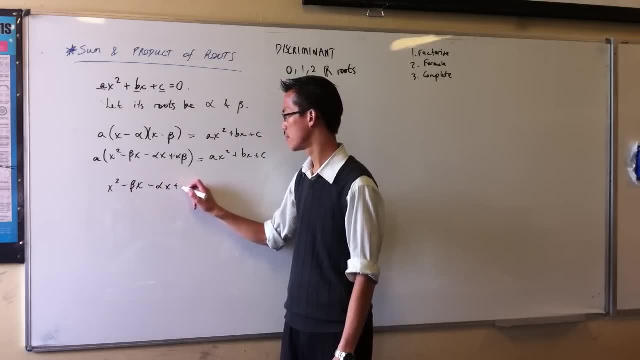 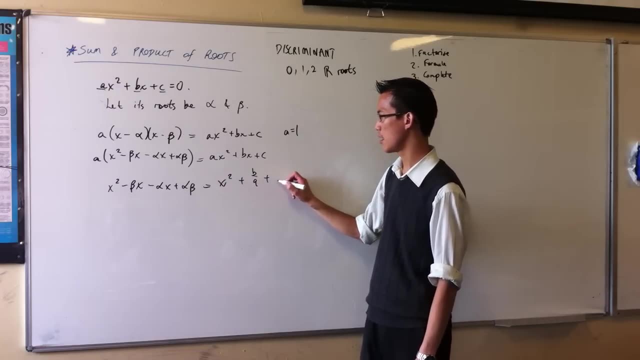 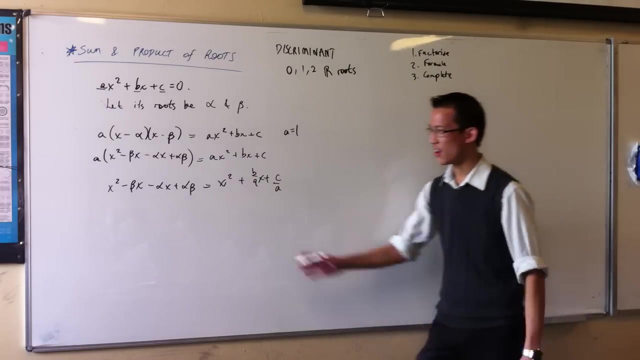 So I've got this, And if I'm dividing everything by a over here, this becomes monic, this becomes b over a, x and this becomes c over a. Divide every term, yeah, Okay. now what's happening over here, on the left-hand side? 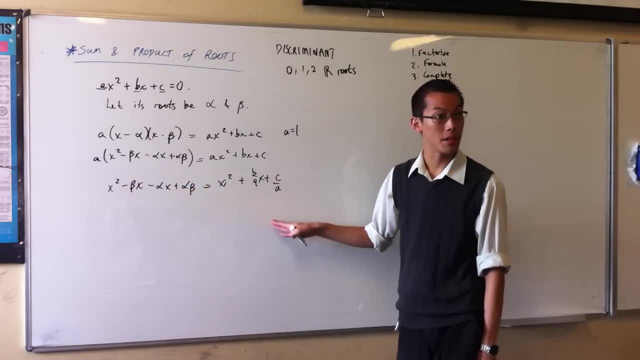 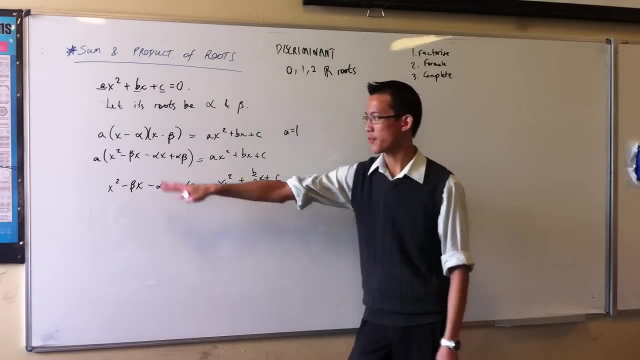 I want to rearrange it so it's more similar to this side. okay, So my x squareds, they're fine. Okay, so I'll just leave them alone. What have I got here? I've got a bit of a jumble. 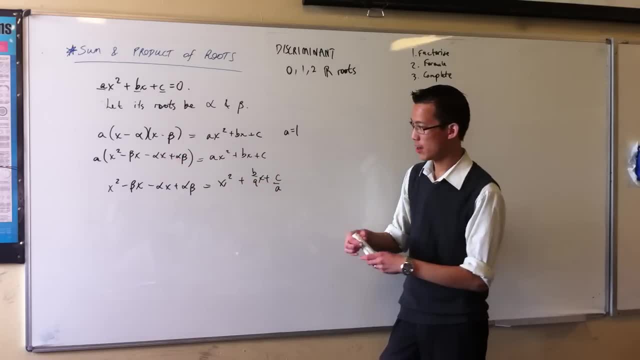 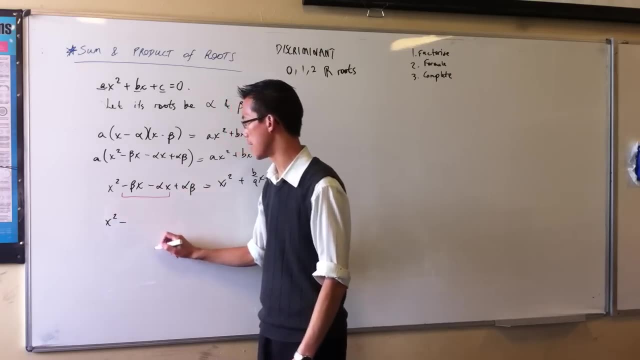 whereas over here I've got it all nice and neat. I've got all the x's together right, So I'm going to take all of these guys and I'll factor out the x, So I get x squared minus. Okay. so what's the double negative? 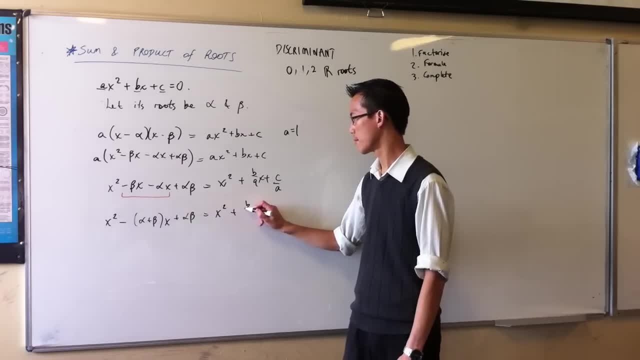 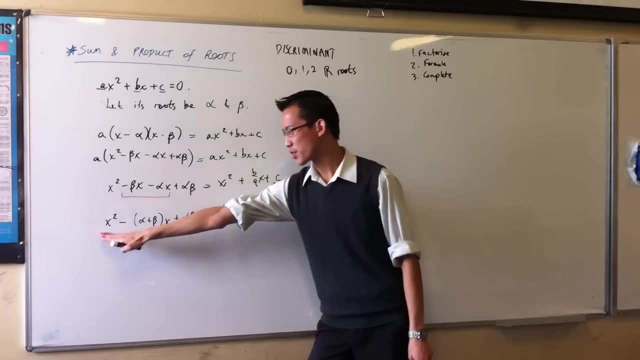 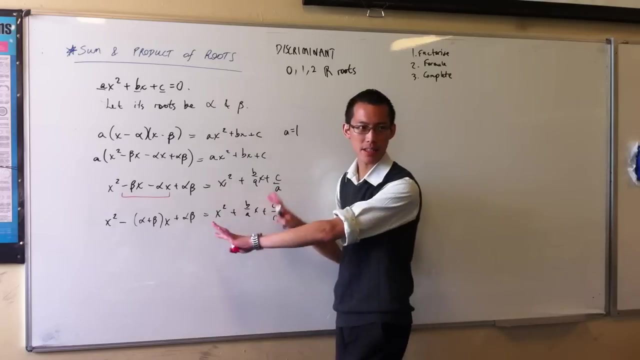 There's my alpha beta. Okay Now, what does this mean? Because I've got all the x squareds here and here, all the x's here and here, and all the constants here and here. they don't mix. It's a bit like oil and water. 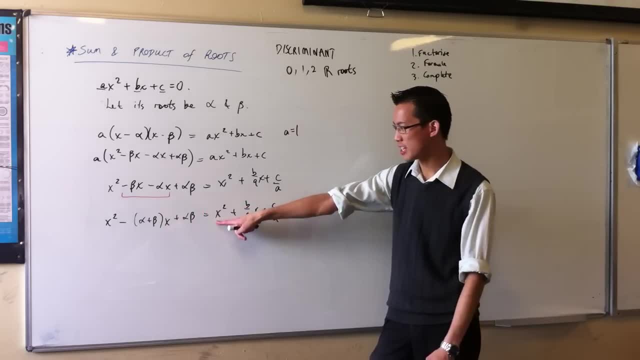 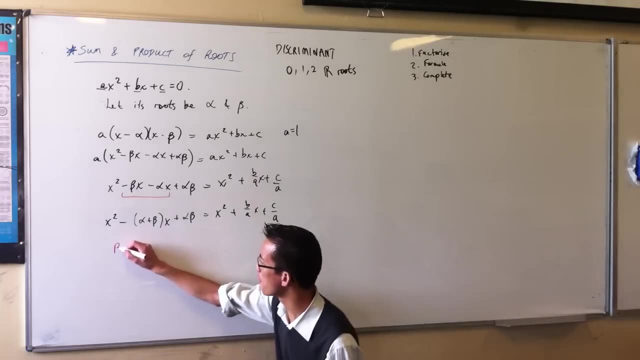 These parts aren't going to magically turn into a constant and these parts aren't going to magically turn into an x, or vice versa. okay, So my next line would be: by comparison of coefficients. You see, that's what I'm doing here. 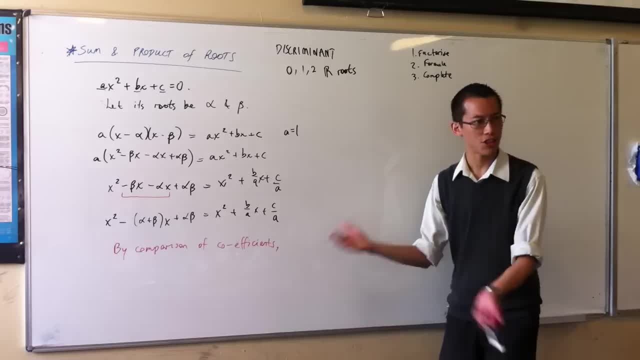 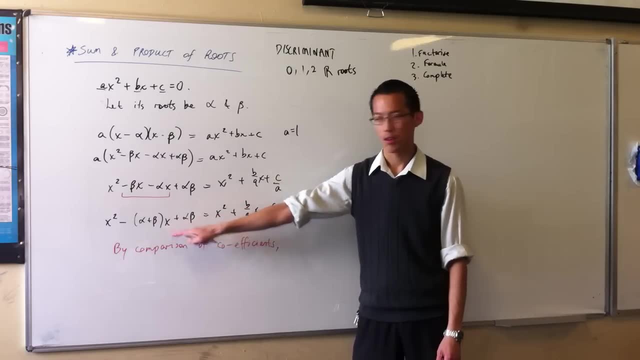 I'm looking at each side and saying the coefficients should match up. I've got x squareds over here, They line up. I've got x's over here, They should line up too right. So minus alpha, plus beta, that's the coefficient on the left-hand side. 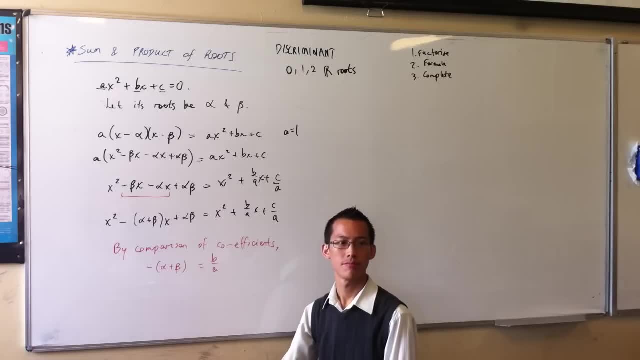 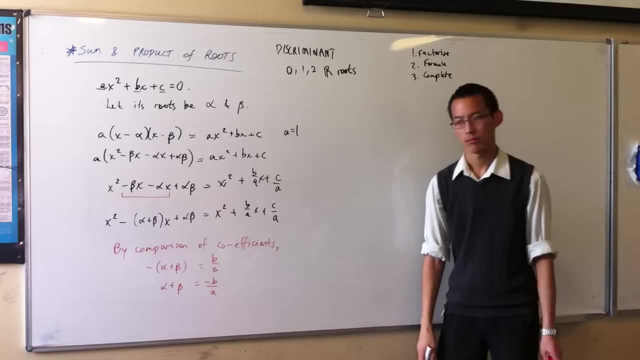 should be equal to b on a. okay, Or perhaps you're more familiar with looking at it without the negative sign on that side. There's the result, okay, And in the same way, just looking at the end here, right, Alpha, beta, the product of the roots. 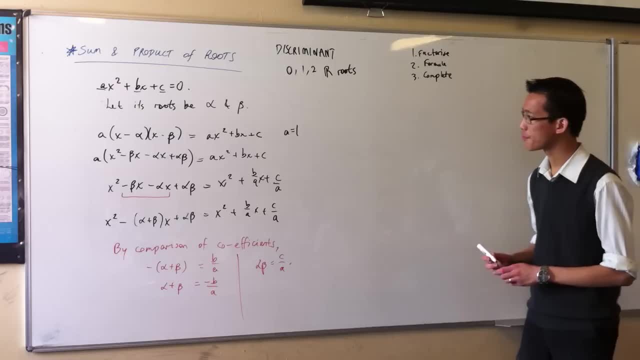 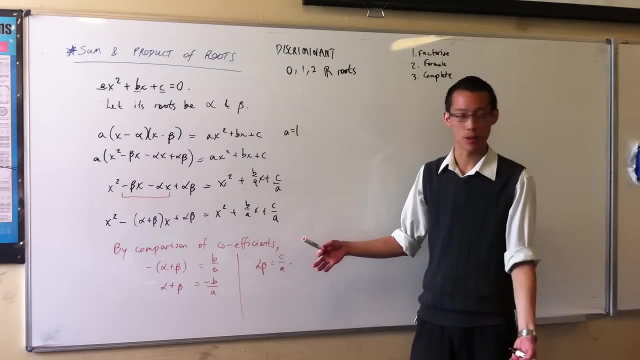 is c on a. Okay, Now, I think that's probably the quickest way to derive these results. It's really simple algebra. actually, You could have probably used half as many lines as I did, but I just wanted to make it super, super obvious. 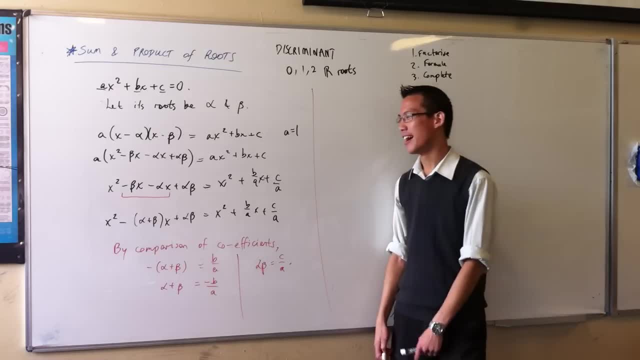 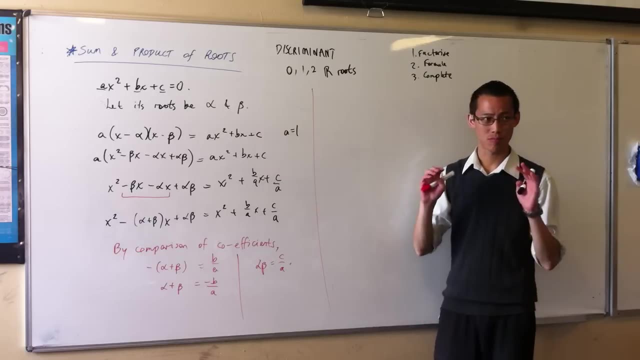 However, you might not like that way, because it seems a bit black magic to me, Like why did you do that? Why did I even start with this line? Okay, So let me show you just quickly. okay, Just so you've got more tools in your toolbox. 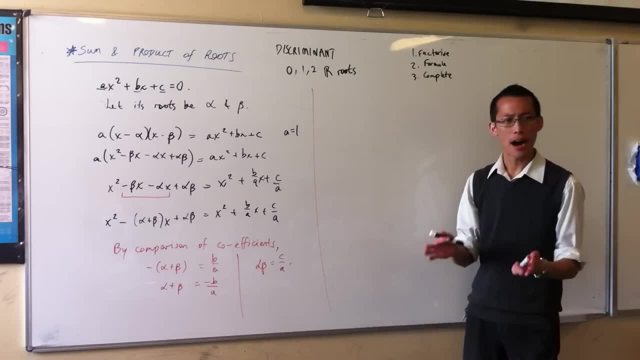 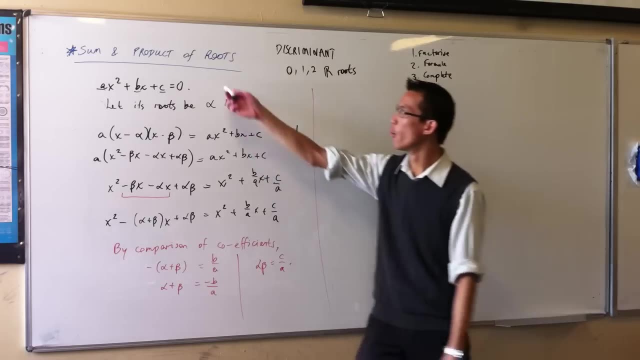 and maybe you prefer this method rather than this one. If I'm after the sum and product of roots, okay, The more direct way to go after them is just to say what the roots are and then add them up. That'll give you the sum right. 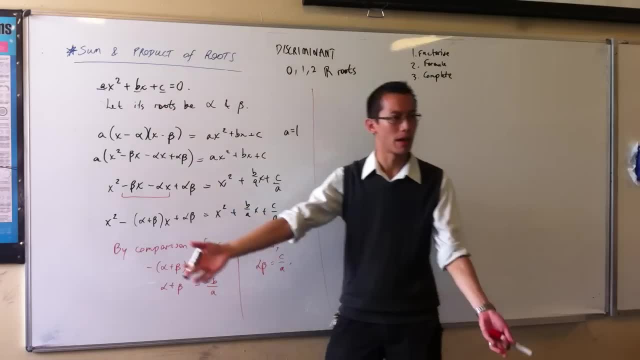 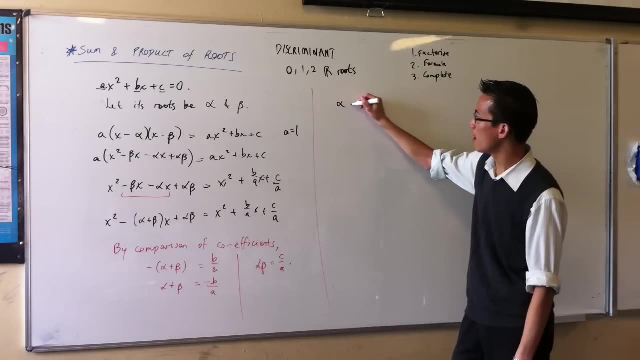 And then say what the roots are and what's the product. Multiply them okay. See what you get right. So if I've got alpha and beta, I actually know what their values are. Alpha would probably be equal to this. 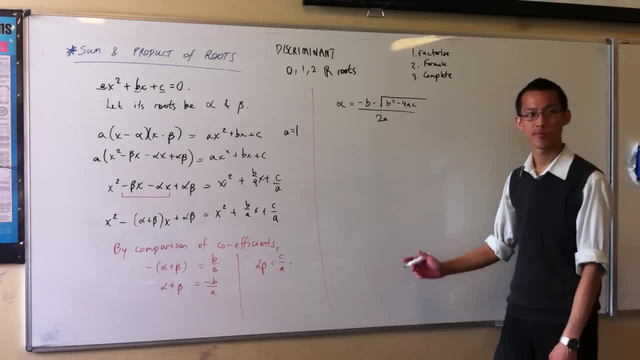 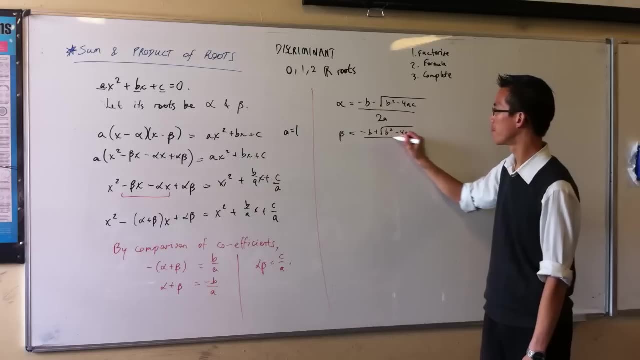 That's one of the roots, isn't it? What's the other one? It's just with an addition. right, It's the conjugate, if you like. Okay, Now, if this is one root and this is the other, 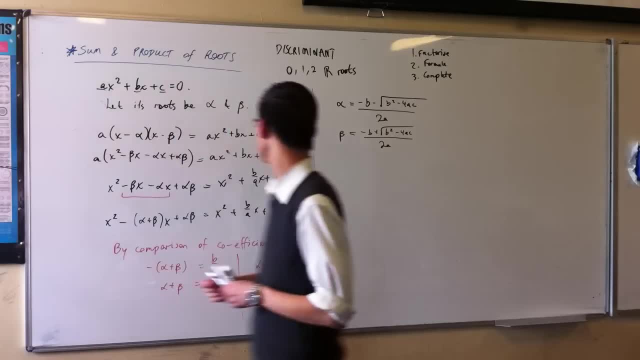 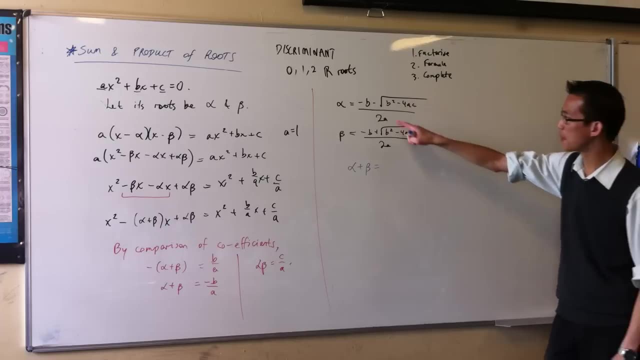 what is the sum? What's the sum? You're looking at it at first and you think that's really gross. I'll look at all this business, But actually when you add them up because of this negative and this positive, that's going to cancel right. 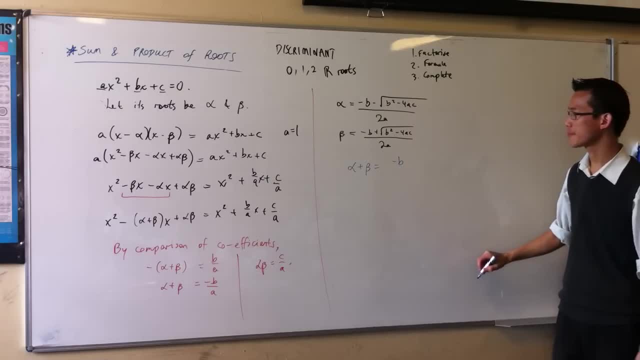 The disgusting part. So I'm going to get minus b and minus b. that's the two parts that actually count, right, All over the same denominator. yeah, Minus 2b over 2a. Oh, that looks kind of familiar, right. 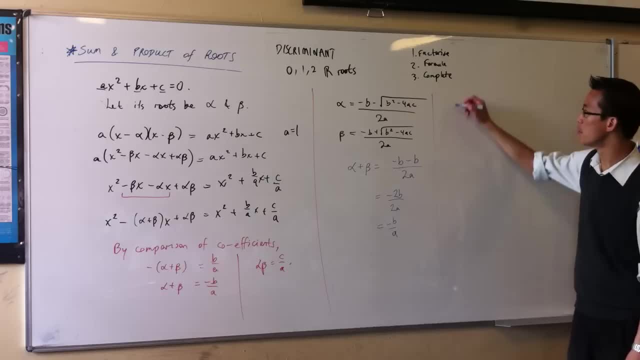 I'm just adding up the roots. In the same way, if you multiply the roots again, it looks as if it will be very bad right, As if it will come out terrible numbers, terrible letters. sorry, But because they're conjugates. 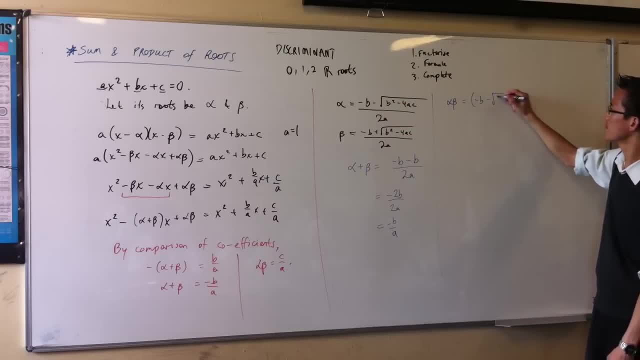 because they're conjugates. this is actually a factorization you learned all the way back in year 8, or it might have even been year 7.. There's one, there's the other. 2a times 2a, it's just multiplying through, right. 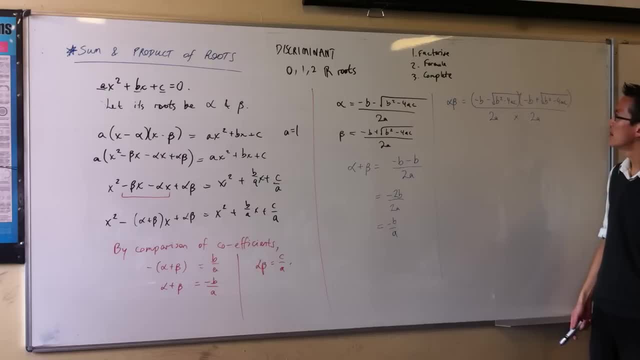 What's this thing on the top here called? What is that? This is the difference of two squares, right? I know it's confusing with the a's and b's, but this is a minus b and a plus b, right? So the result should be a squared minus b squared.